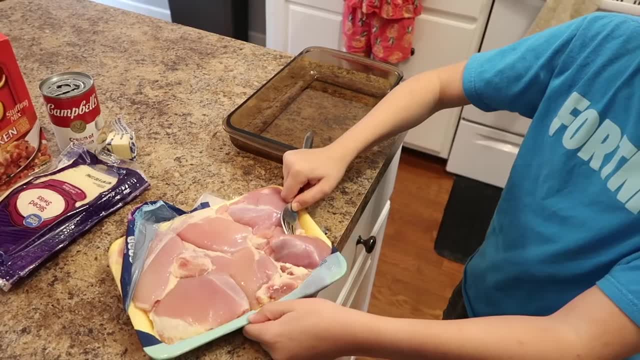 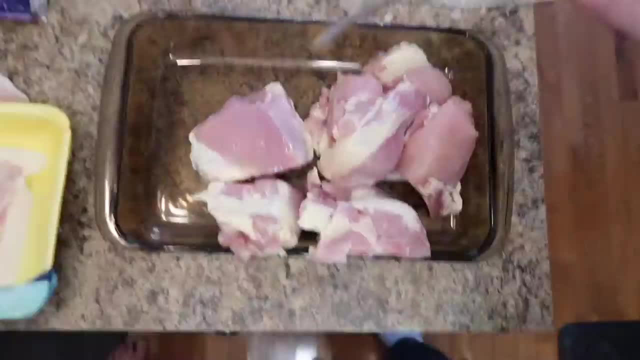 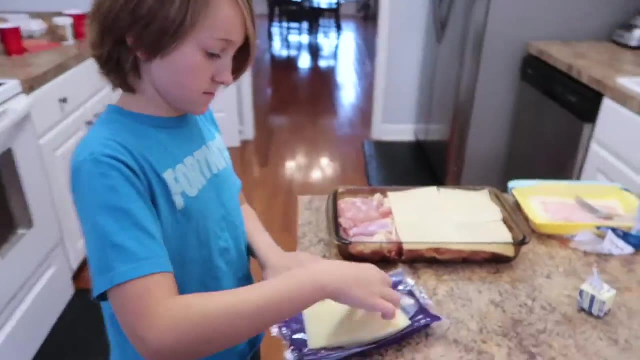 you like stuffing, butter, milk and cream of chicken. So you just put six chicken thighs into your 13 by 9 casserole dish And then you cover the chicken with one layer of cheese. Then you need to mix up the cream of chicken. Can you take the milk? 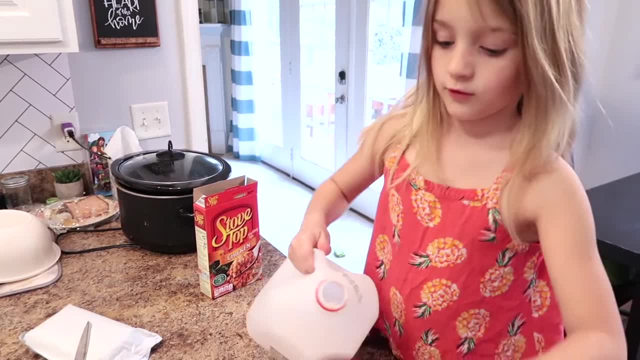 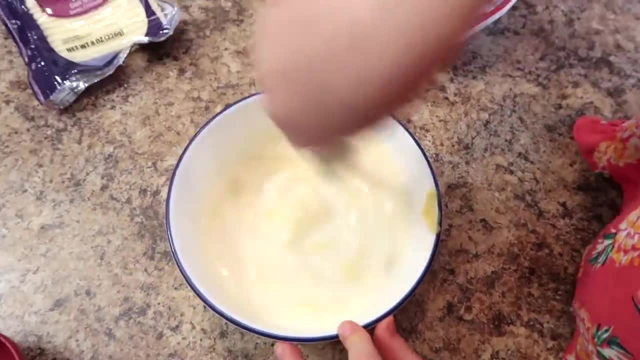 How much do I put? You're going to need a half cup. Good job, Now can you stir that up? Stir that together until it's blended up. See how it's blending. We're going to pour the whole bowl in. 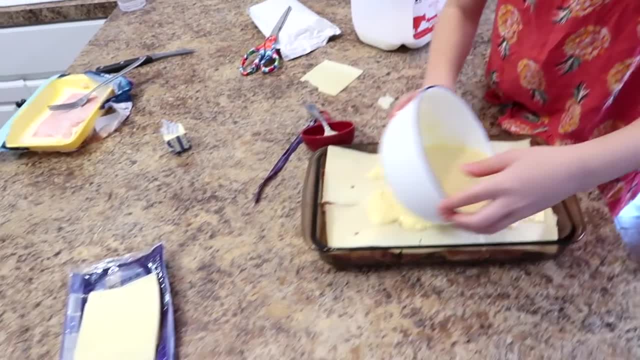 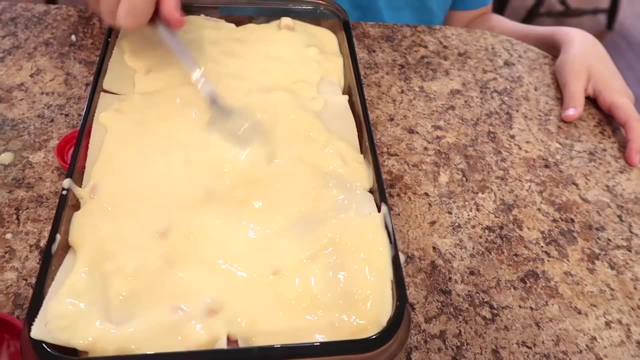 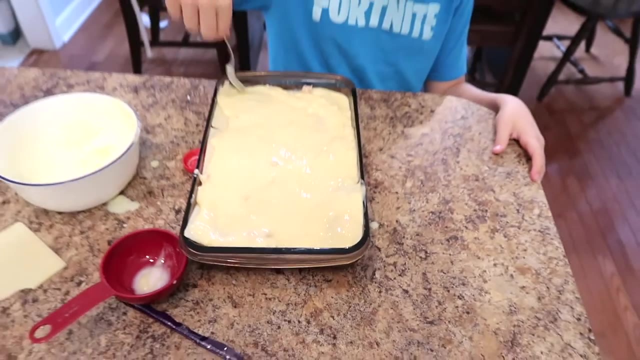 There you go, Keep going. Alright, use the spoon and spread it over top of all the cheese. You can't really mess this up, but we just want to try to get it evenly spread over the top. You're doing a great job, Excellent work. 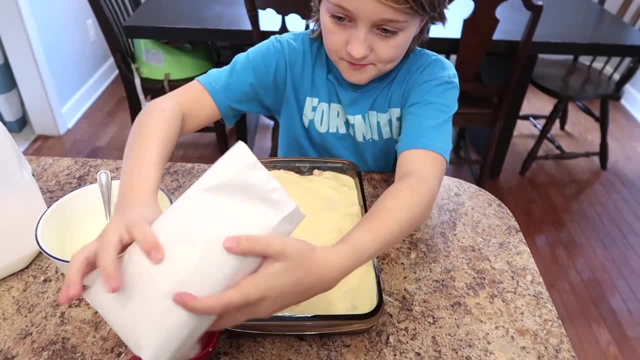 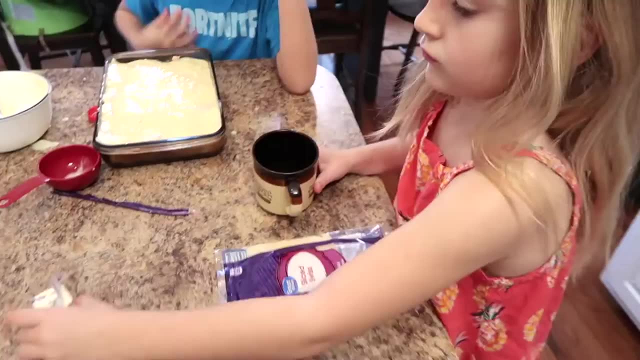 Alright, so you're going to sprinkle the stuffing all over the top. I'm just kind of mixing this up, of want to get it evenly over the top, all right, so now you're going to put the butter into a coffee cup so we can melt it in the microwave. now you're going to pour the melted. 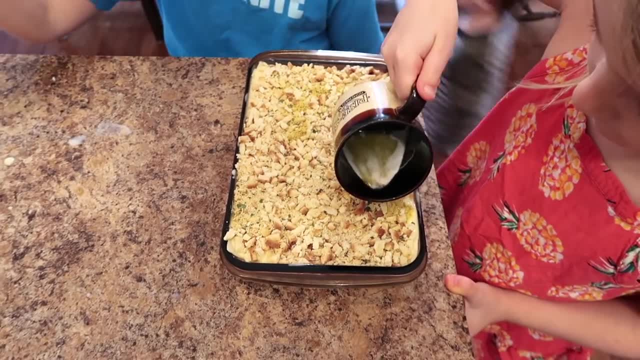 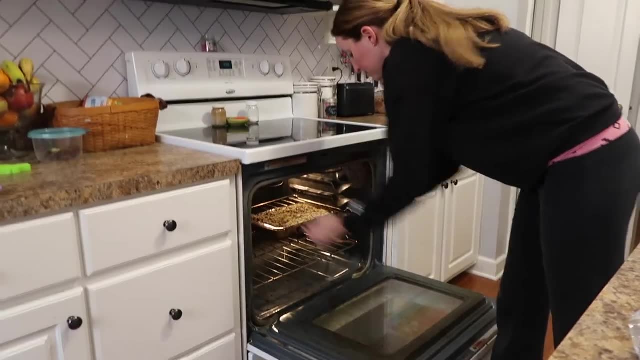 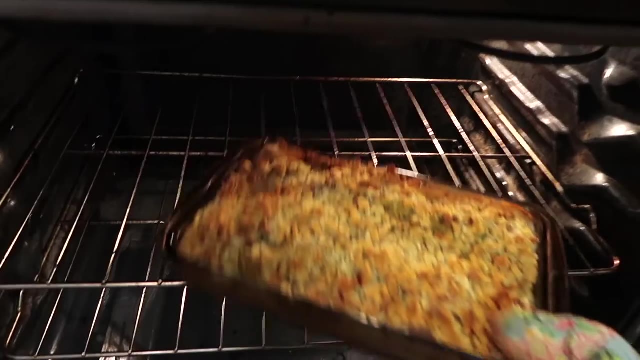 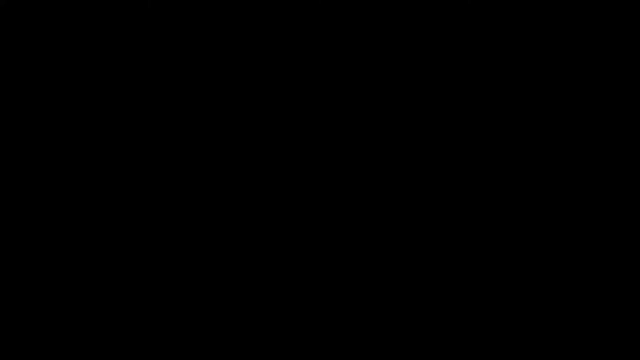 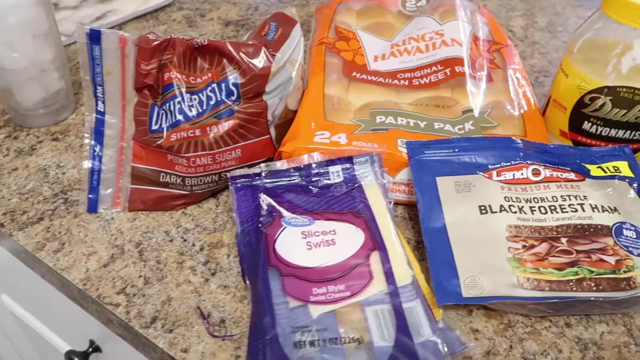 butter evenly over the top of the stuffing. good job. bake it at 350 for 45 minutes. so hawaiian sliders are a fan favorite over here. they're kind of rich and heavy so we don't make them very often. so it's definitely a big treat when we do. 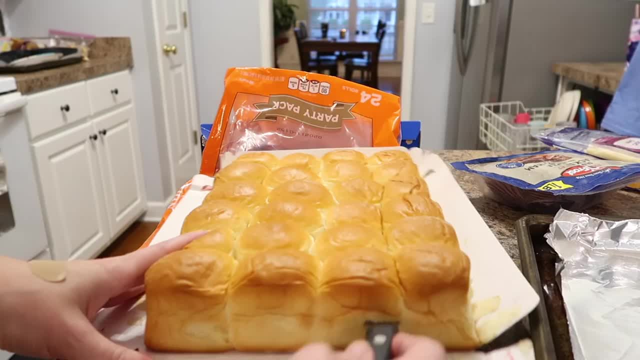 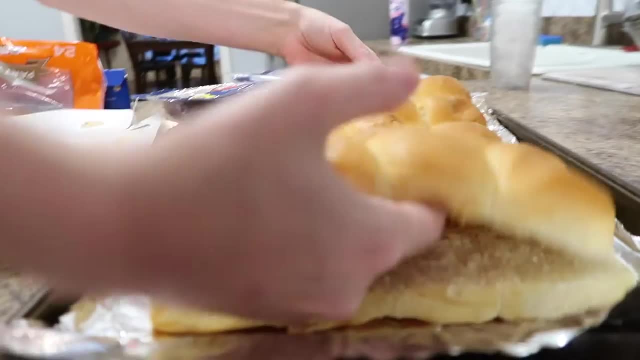 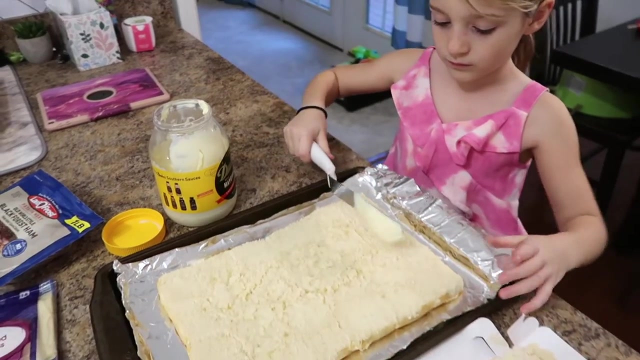 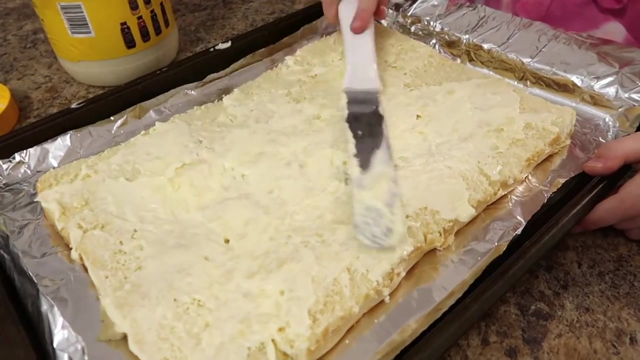 to make this quick and easy, we just cut the whole thing of sliders in half. we'll put the bottom of the rolls on the pan that we're going to cook it in and take the top off. then you spread mayonnaise on the rolls. while one person is handling that job, the other person can come help make the sauce. 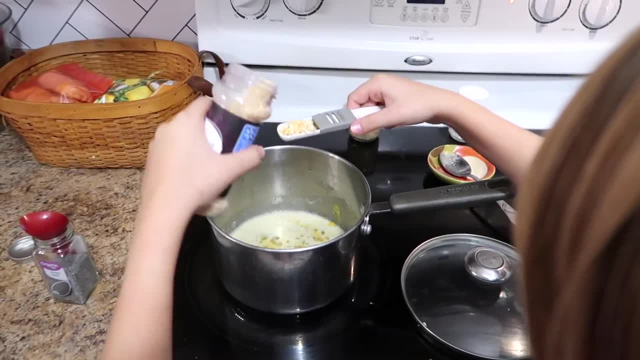 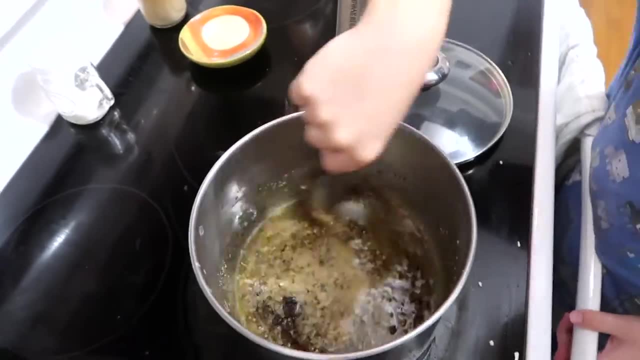 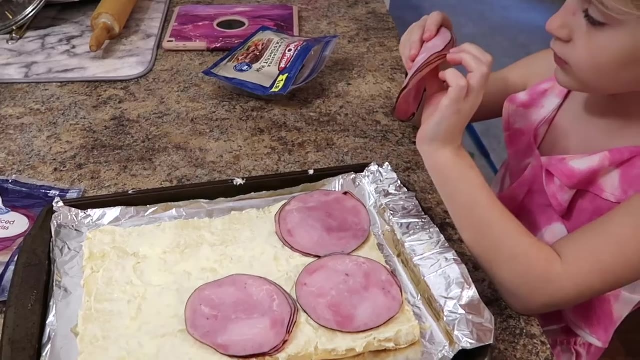 and all the amounts for each ingredient are listed below, either in the description box or there will be a link to a recipe. our secret ingredient, the brown sugar: stir it all together. while we were working on the sauce, my daughter was putting the ham and the cheese onto the rolls. we like to layer our ham three slices high. 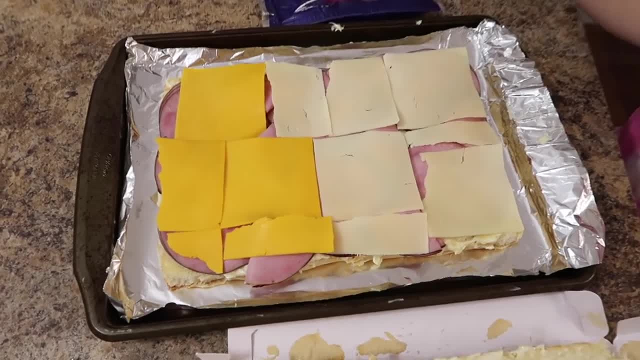 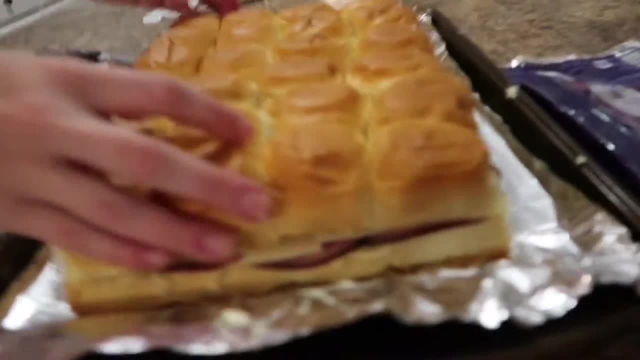 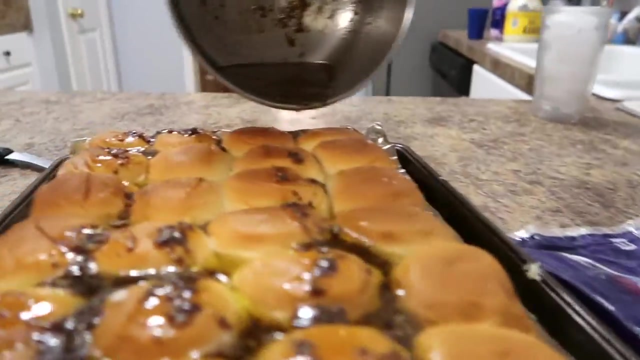 and then one layer of cheese. well, we ran out of swiss cheese, so we used some cheddar cheese tonight, and it was really good too. then you pour the sauce over top of all of your rolls, cover it in aluminum foil and bake it until it's browned. 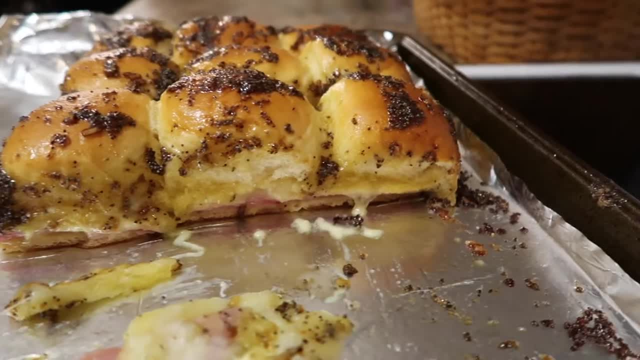 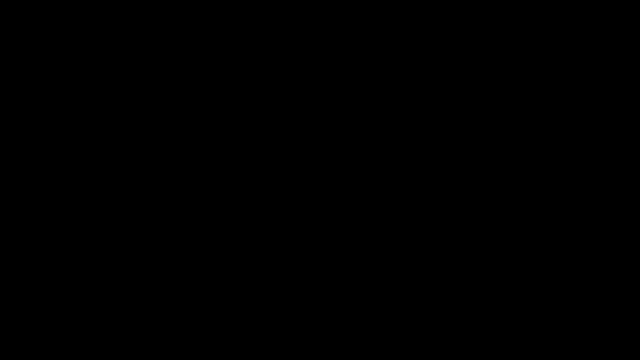 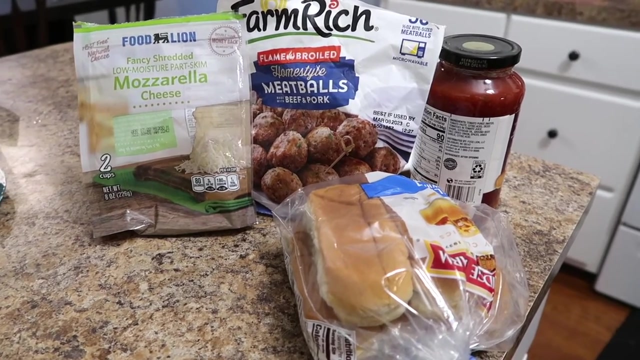 at 350 for 20 to 25 minutes. I'll use a pizza cutter to slice them into individual sliders. Here's a recipe that my older kids can make completely on their own without my help, because it only requires the microwave. All you have to do is microwave your meatballs for a minute. 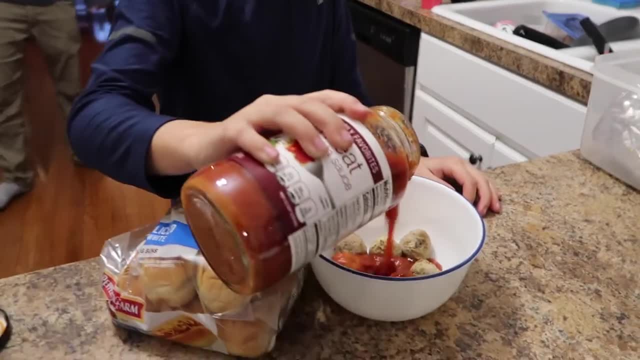 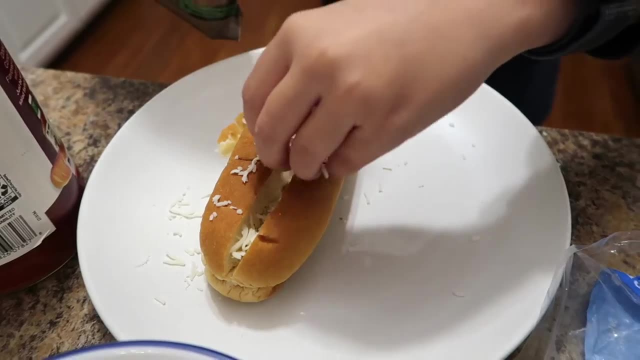 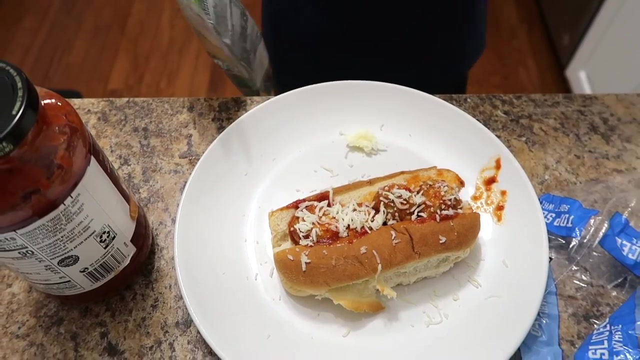 take them back out, pour some sauce over top and then microwave them for another 30 seconds to a minute, depending on how many meatballs you're making. Put some cheese into your roll, put the meatballs on top, top those with a little more cheese and voila, Dinner is served. 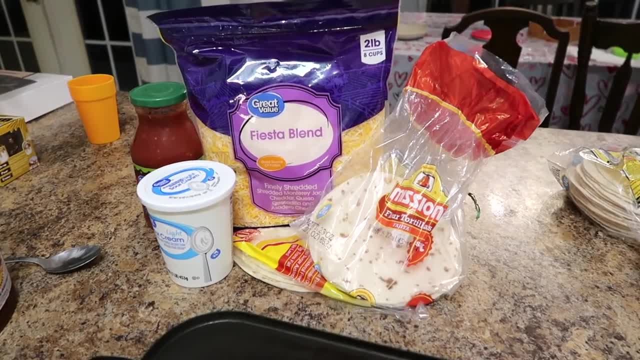 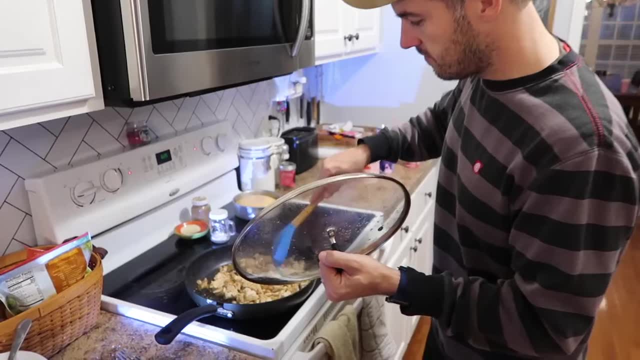 You just need tortillas, chicken, taco seasoning, cheese and anything else you like to add to your quesadillas. So, of course, one of us will make the chicken and we season it with some taco seasoning. We like to use our griddle for this. 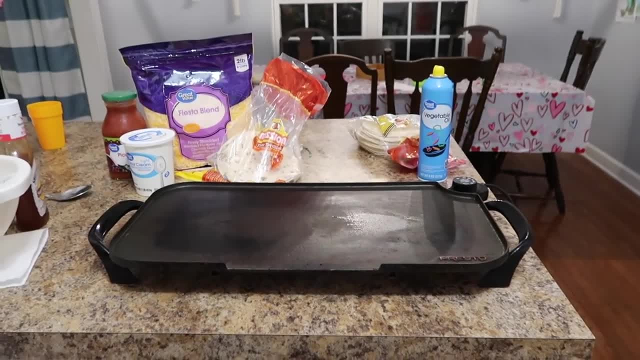 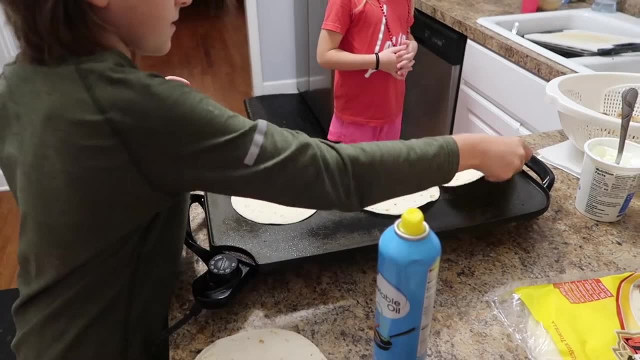 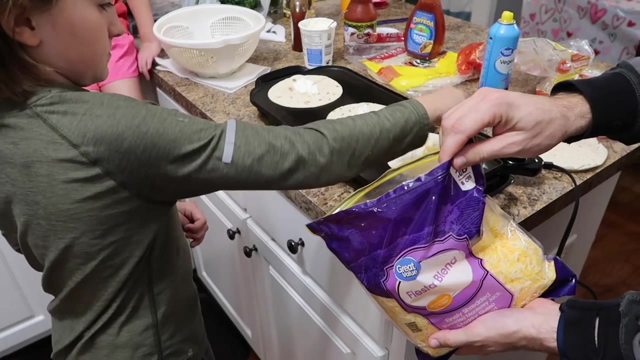 We have four kids, so with a family of six we're obviously making a lot of quesadillas, so this makes it go a lot faster, And we're using small tortillas so we can fit three quesadillas at once on our griddle. Now the griddle is pretty hot, so we are watching carefully and only letting our older two 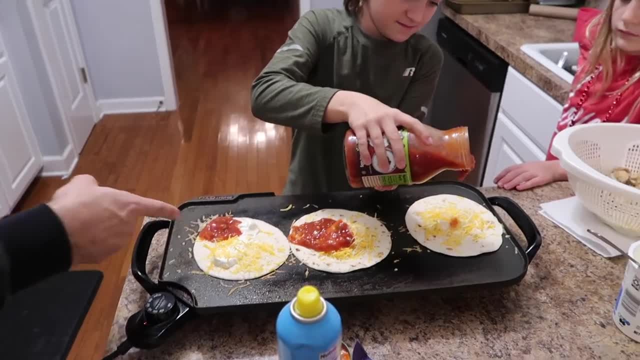 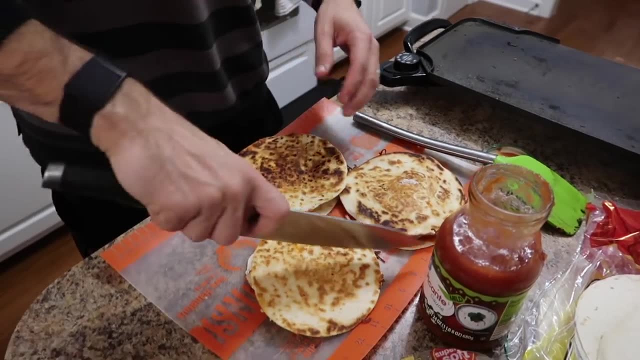 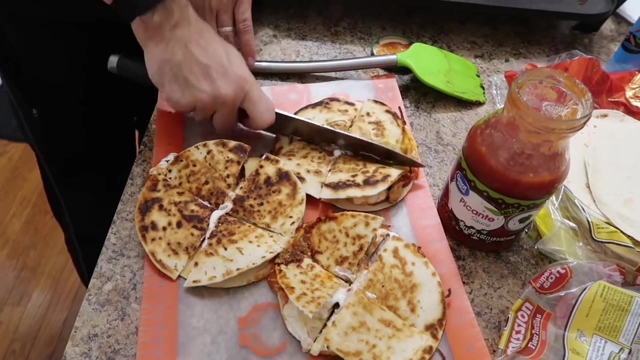 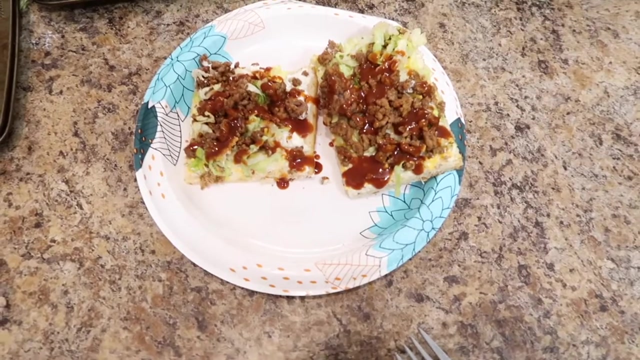 help with this job, And then my husband or I will be the ones doing the flipping of the quesadillas to cook them on both sides, And then we just cut them into quarters and they're ready to go. This is one of my favorite meals. It's so easy and I really enjoy these leftovers for lunch. For this meal you'll need: 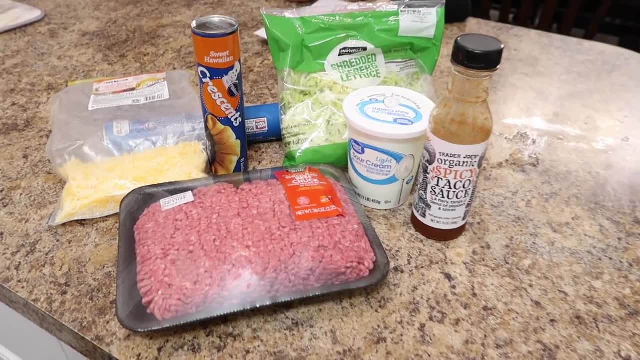 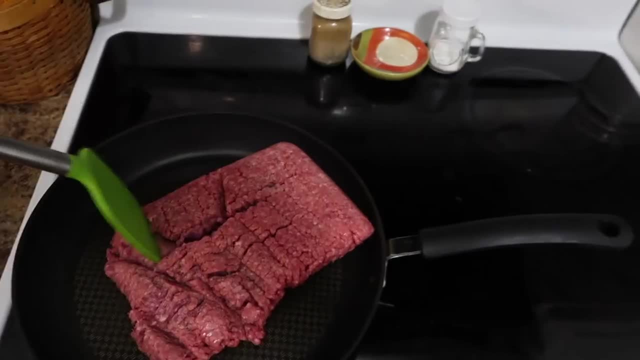 ground beef, crescent rolls, cheese, shredded lettuce, sour cream and we like to have some taco sauce on ours. I will cook the ground beef and season it with some taco seasoning. I will cook the ground beef and season it with some taco seasoning. 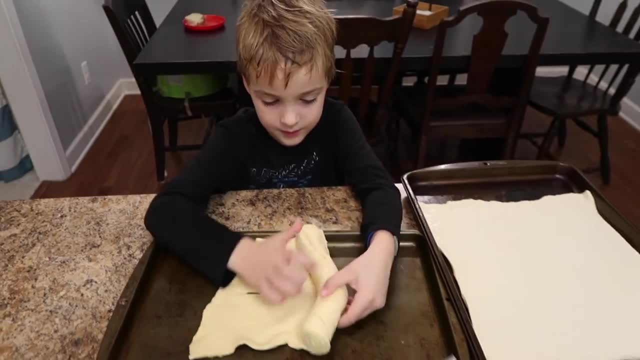 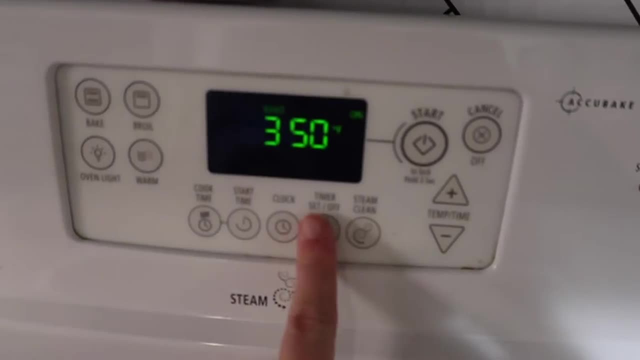 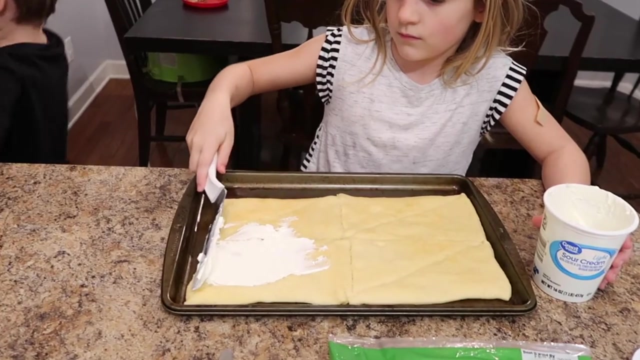 And while that's cooking, my five-year-old can actually roll out the crescent rolls onto the pans, And then we can have that cooking while the beef is cooking- And so usually they're done about the same time- And then your kids can spread sour cream all over the top. 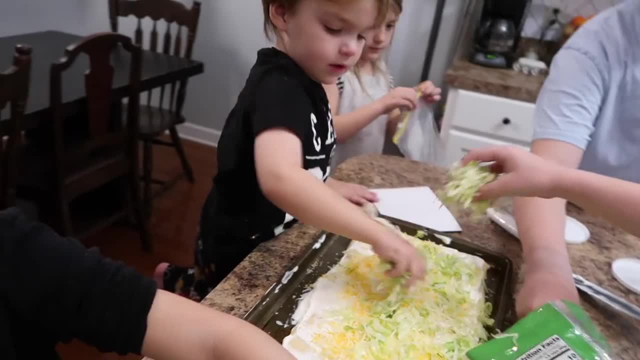 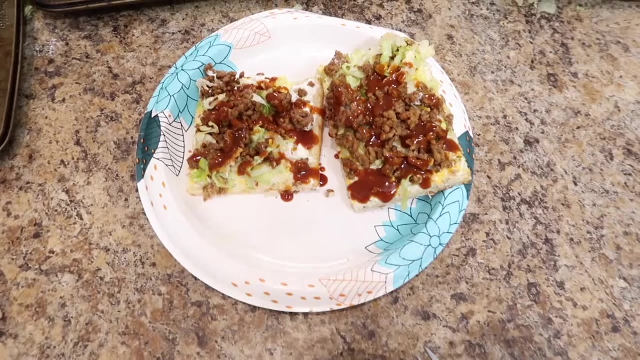 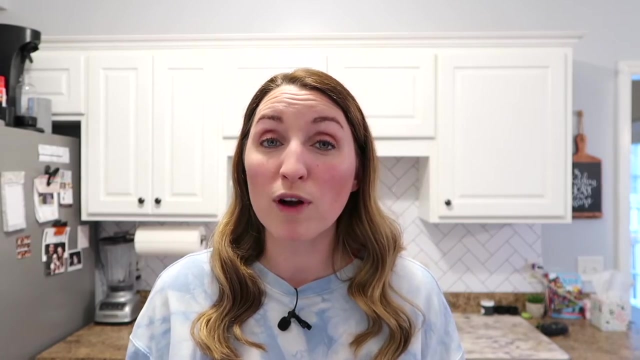 Then sprinkle some cheese on And then sprinkle the shredded lettuce And then sprinkle the ground beef over top, And then I'll just let whoever wants taco sauce, they can put it on their own pieces. I love having a list of easy meals that I can pull from when I'm planning out my menu for the week. 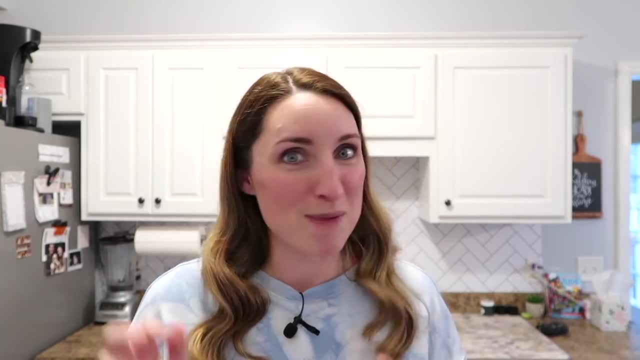 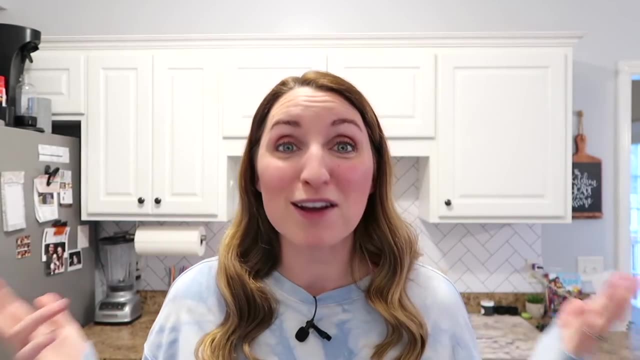 So if you have any other go-tos, please put them in the comments below for me and everybody else watching, so we can all share some great ideas together. Hopefully this will help you plan out your next menu and get you set up for the next week or two of easy meals. 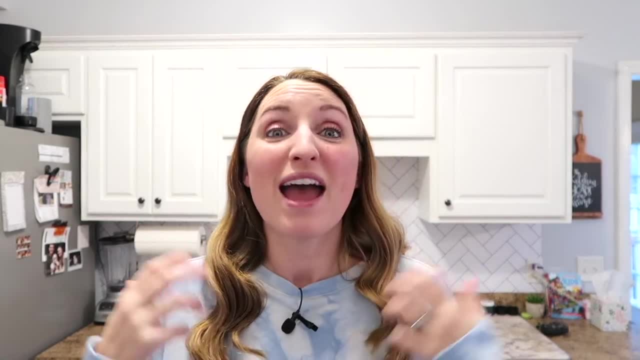 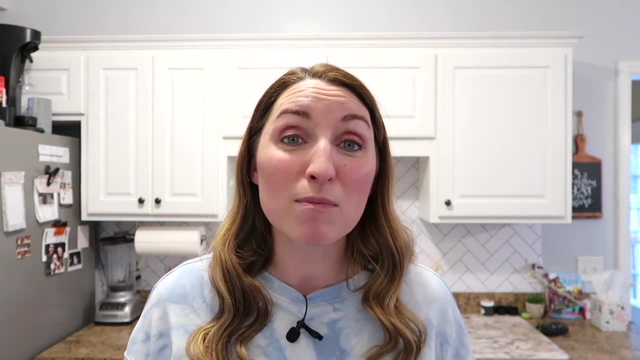 And hopefully your kids will enjoy making these with you And y'all can cook And create some beautiful memories together without you wanting to pull your hair out. My name is Sarah and I'm a homeschooling mom to four kids, And my channel is all about homeschooling and life as a family of six. 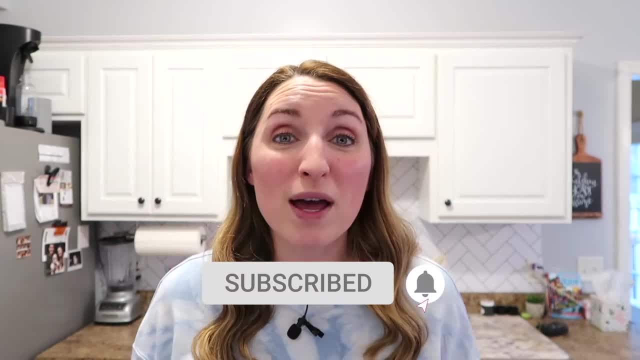 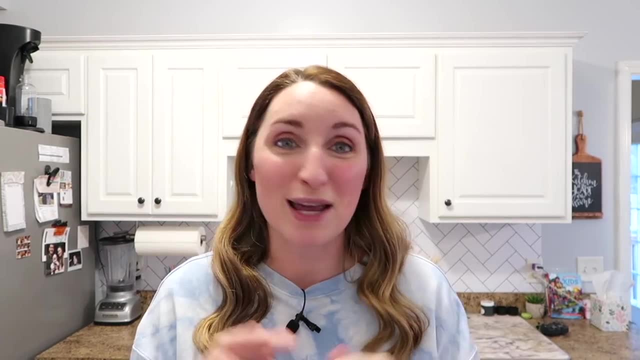 So if that interests you, go ahead and hit that subscribe button below. This year I'm posting every first and third Wednesday of the month, So hit that little notification bell so you don't miss another video. And if you enjoyed this video, please give it a thumbs up. 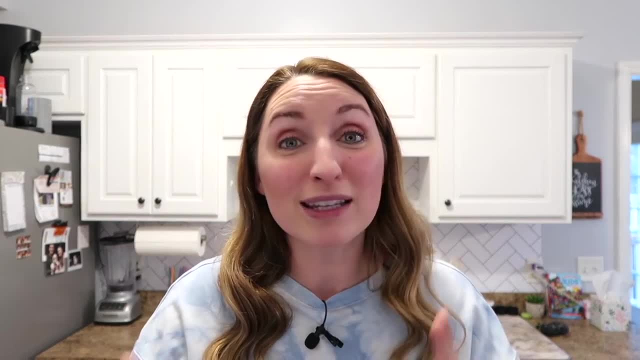 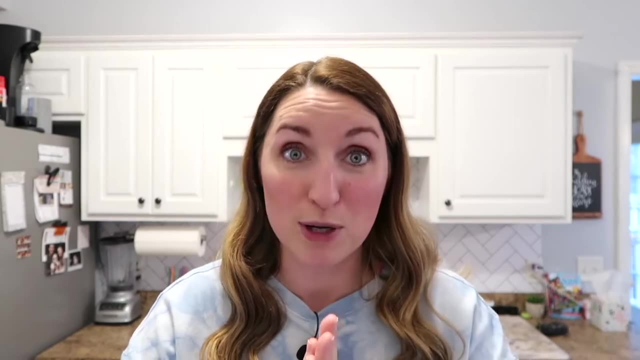 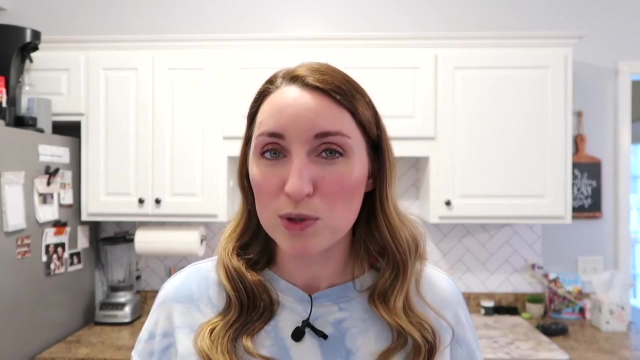 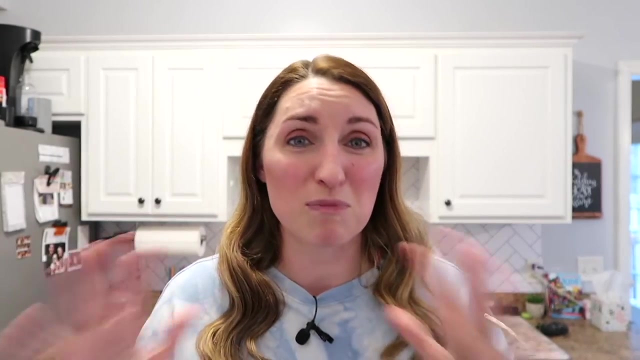 That really helps the video. I also wanted to share with you that I just recently launched a new business that's for you moms. It is a party in a box subscription box. I'm super excited about it. So if you remember having holiday class parties in school but now you homeschool and you want your kids to have that experience but you don't feel like adding another thing to your plate. you don't want to do all the interesting and the planning and the going to all the stores and get all the things. 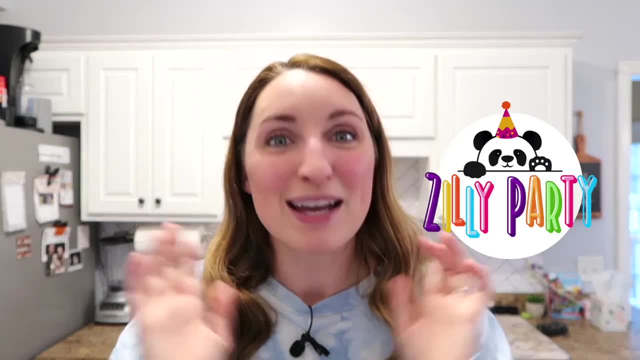 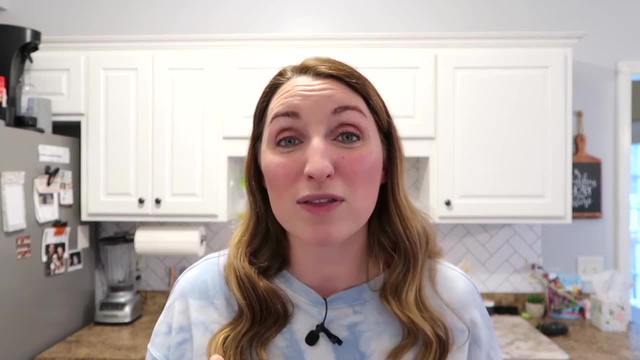 I have the solution for you. It's called silly party, So after this, go check out the link below And you can get 20% off your first box. It's six holidays throughout the year: holidays and celebrations- Like we've got a end of the school year celebration box.